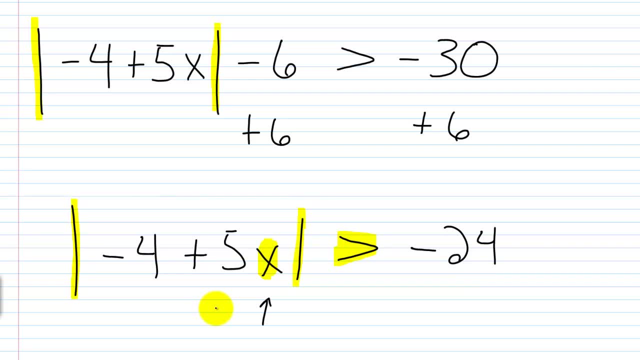 four. If it's zero, take the absolute value. you'll get zero, that's greater than negative twenty four. and if it's positive, take the absolute value. it's still positive, that's greater than negative twenty four as well. So, no matter what, you'll always get a true. 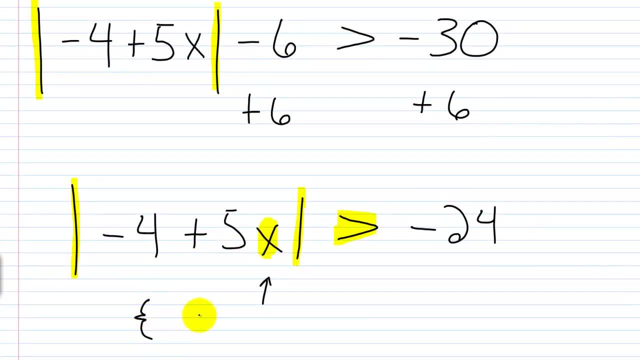 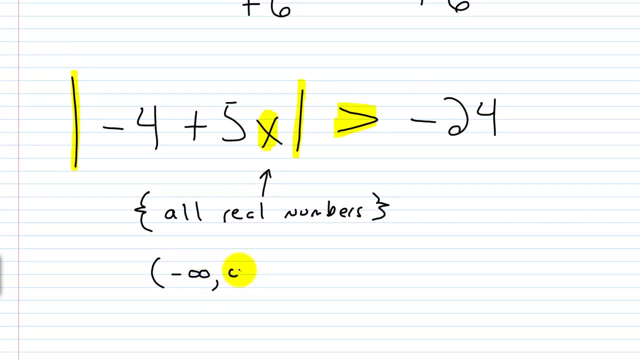 statement and when we come across something like this, we basically say that your solution would be all real numbers- and you could say it like that- or an interval notation. okay, you could basically put from negative infinity to positive infinity, because anything would work. Then we have a number. 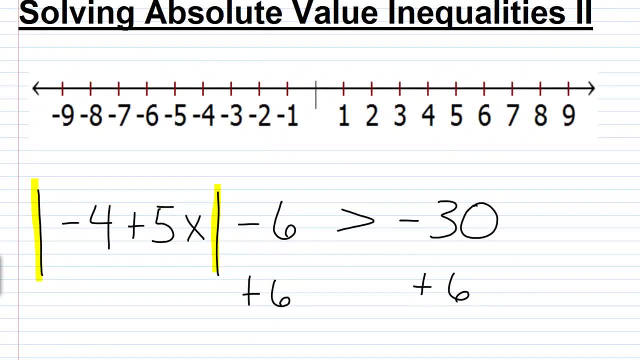 line so we could kind of graph it. and if we wanted to graph it, basically what we would say is that I would just shade the entire number line, I would just shade everything on that number line. Make sure you shade those arrows to indicate that it continues indefinitely in both directions. 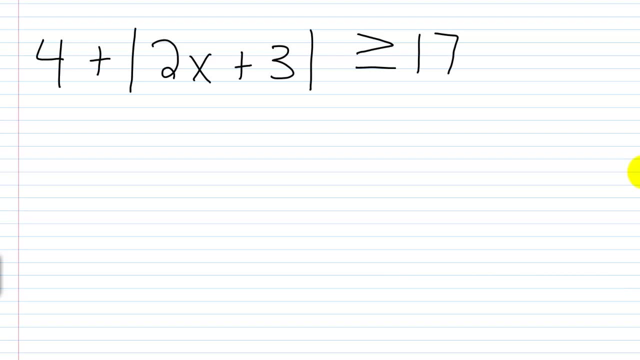 Okay, let's take a look at another problem here and here we have four plus the absolute value of two x plus three is greater than or equal to seventeen. So our goal is always to isolate this absolute value part to start. So I'm just going to subtract four away from: 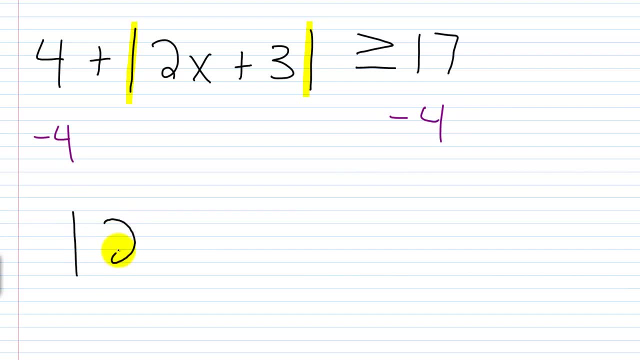 each side to make that happen, and we'll have the absolute value of two x plus three. and then we'll have the absolute value of two x plus three is greater than or equal to seventeen minus four is thirteen. So now let's think about what to do here. If you watch the main, 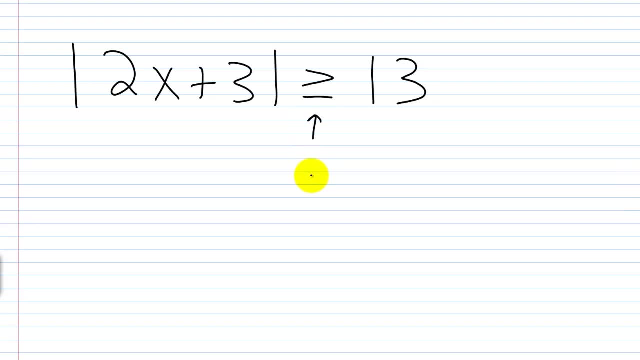 lesson. you know that whenever you have a greater than, or greater than or equal to, it sets up into this or scenario, You have this compound inequality with, or The first one. you basically just remove your absolute value bars and you write what's there, So you'll have two x plus three is greater than or equal to the number thirteen. 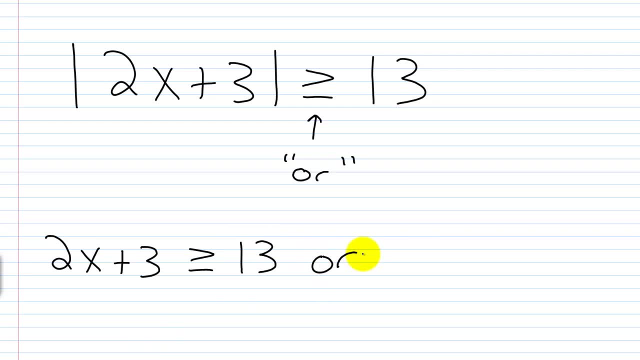 Okay, so that's the first scenario. Then you have, or basically you'll have, remove the bars, so two x plus three. You will flip this sign, so, instead of it being greater than or equal to, it will be less than or equal to, and then you'll make this negative. So this will become: 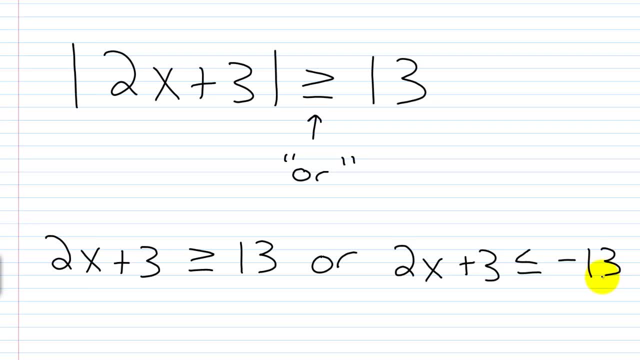 negative thirteen Because, basically, if the result of this- I pick some number for x, I plug it in- I multiply it by two, I add three, If the result of that is less than negative thirteen, Think about what happens when you have a negative thirteen. Think about what 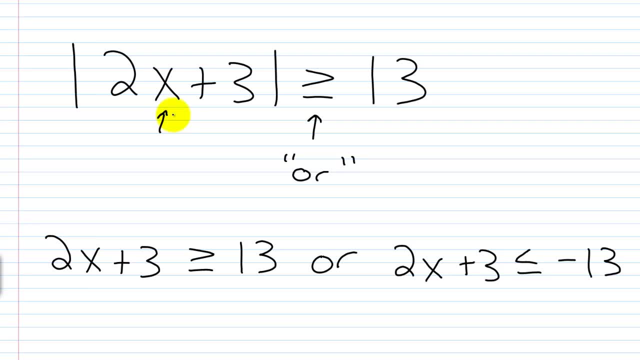 happens when you take the absolute value. Let's say, you get negative fourteen in there. as a result, You take the absolute value of that, you get fourteen, And fourteen is greater than thirteen. so that works out. So, basically, that's why you have these two scenarios: This: 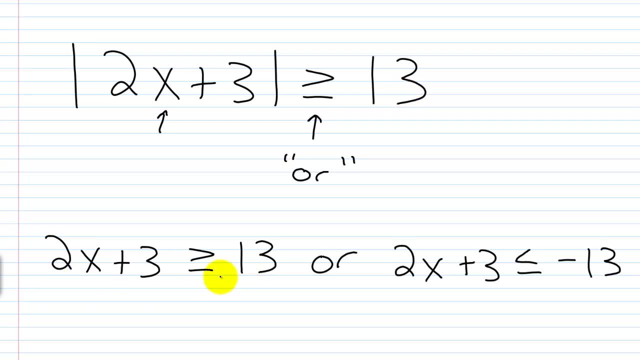